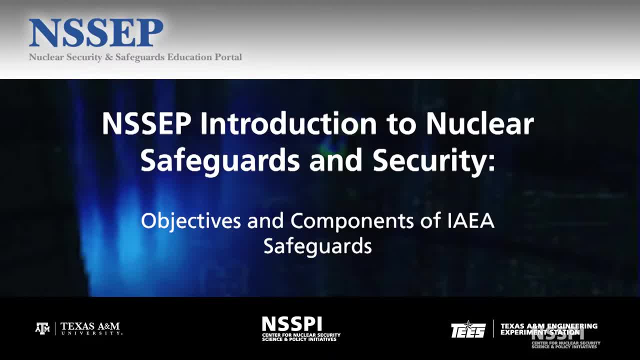 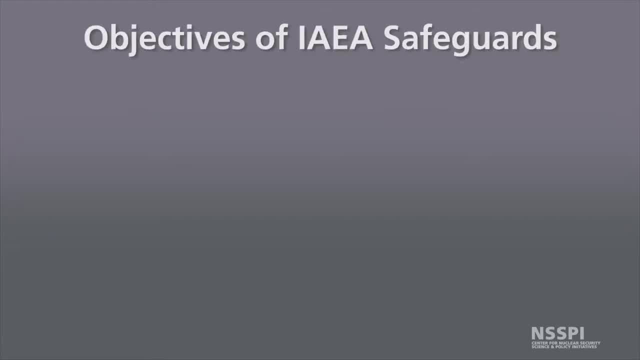 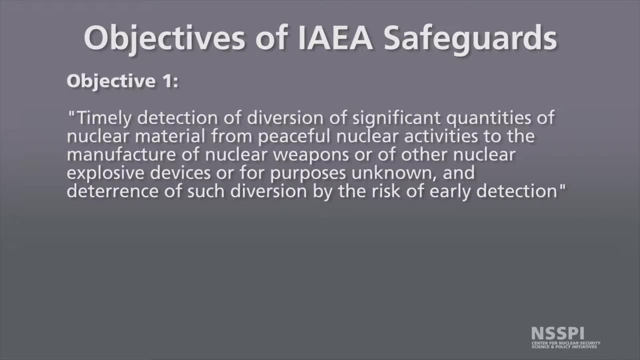 So the objectives of IAEA safeguards if we take a little closer look, the first objective is timely detection of diversion of significant quantities of nuclear material from peaceful nuclear activities to the manufacture of nuclear weapons or of other nuclear explosive devices or for purposes unknown, and deterrence of such diversion by the risk of early detection. 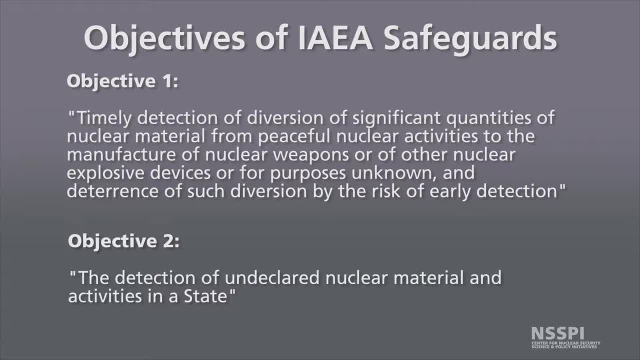 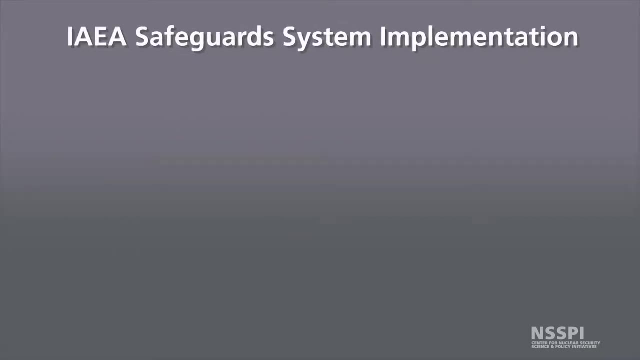 The second objective is the detection of undeclared nuclear material and activities in the state. So those two objectives work together to prevent further proliferation from civilian nuclear programs. So now let's take a look at IAEA safeguards system implementation And the four general phases of safeguards system implementation. 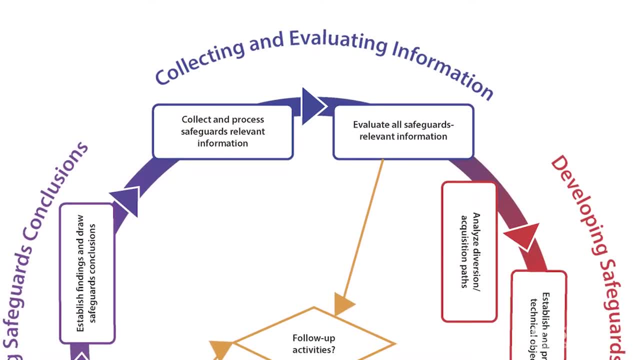 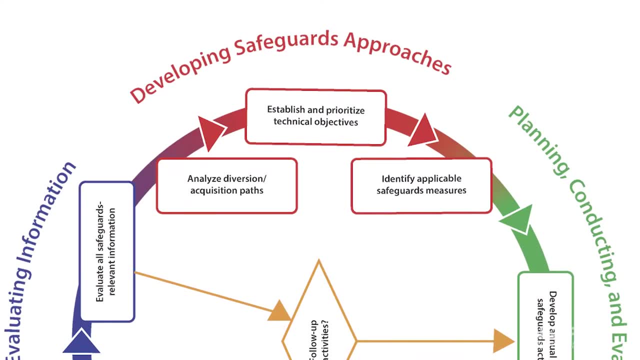 The first begins with collecting and evaluating information- What facilities does the state have, What activities are they conducting? And then, from that information, developing a safeguards approach. How are safeguards applied at the facility or facilities within a state? And then, once a safeguards approach has been developed and applied, 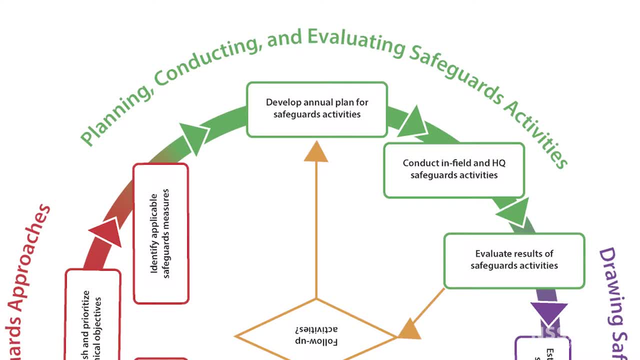 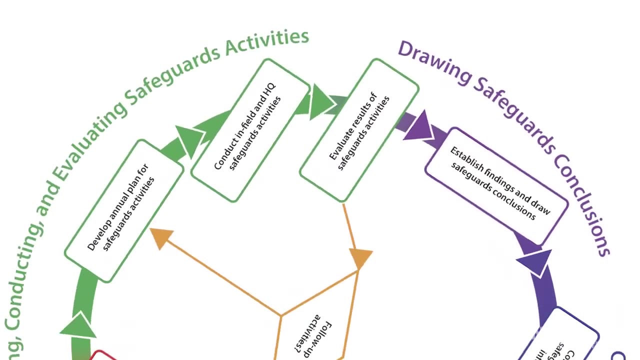 The IAEA can move on to planning, conducting and evaluating safeguards activities, whether that's inspections, other methods to verify the non-diversion and misuse of nuclear facilities, And then from those safeguards activities the IAEA can draw safeguards conclusions: Is the state living up to its treaty obligations and safeguards obligations? 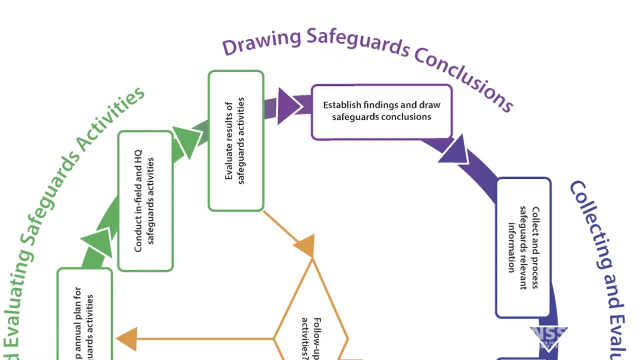 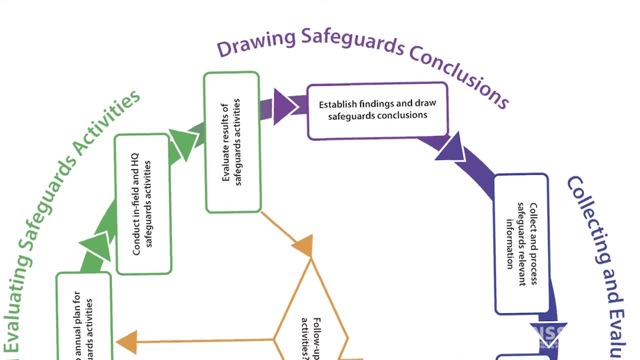 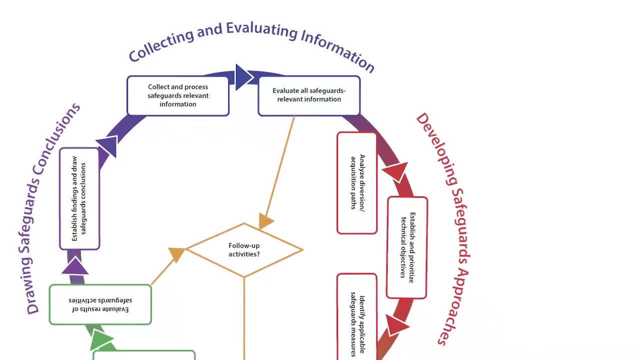 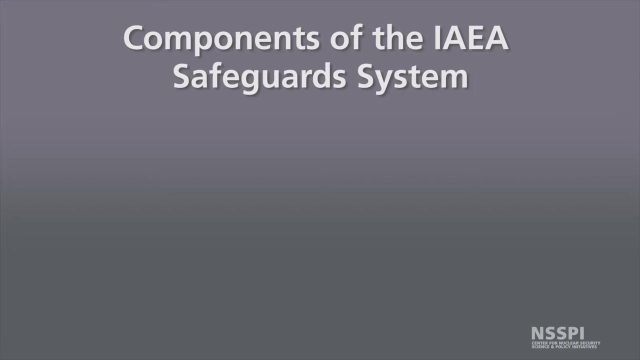 Or is there some non-compliance or some inconsistency? Hopefully there isn't. And then the IAEA goes back to collecting and evaluating information and back through this wheel of safeguards activities of the IAEA, And there are specifically several components of the IAEA safeguards system that the system.